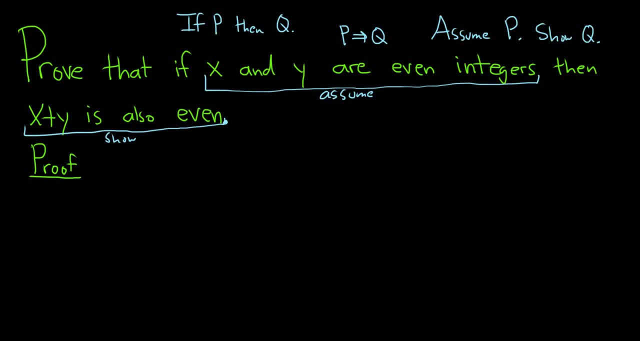 definition of what it means for an integer to be even. So an integer is even if it's a multiple of two. So what does that mean? So we say x is even. This is the same thing as saying if x is equal to, let's say, 2k. 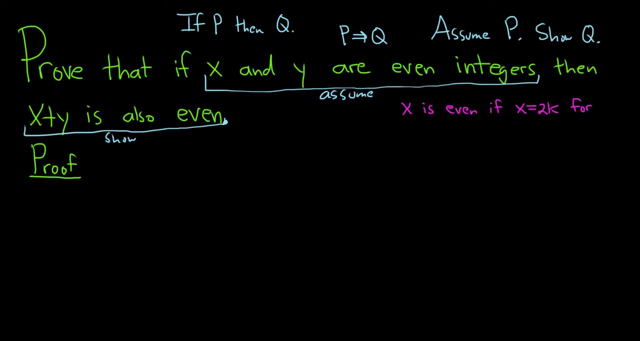 For some integer k. We don't know what k is. We just know that x is equal to two times that integer, So this goes both ways. This is called. it's really an if and only if statement. I wrote if because this is the definition: Definitions. 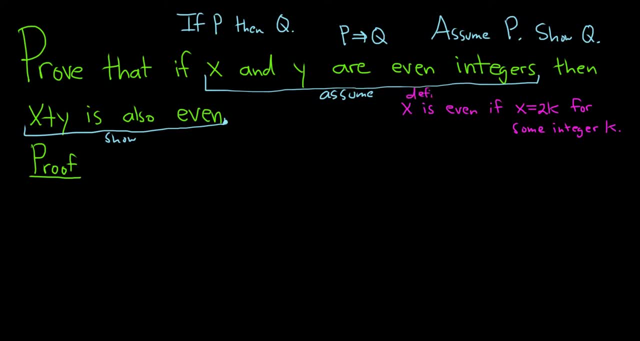 always go both ways. So I'm going to go ahead and put that here. So definition: So, even though it says if it does go both ways. So if x is even, then x equals two k for some integer k. If x equals two k for some integer k, then x is even So. 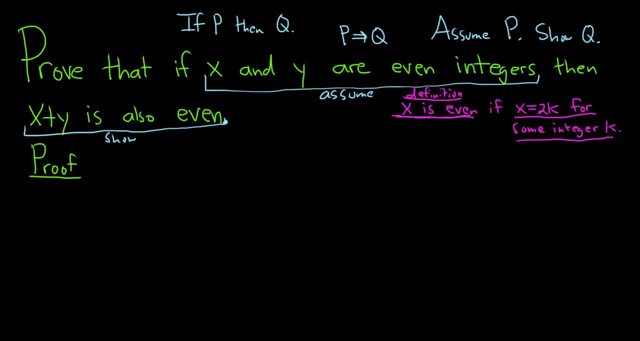 that's what it means for an integer to be even. Okay, let's do this proof. So we'll start by writing down our assumption, our p. So, suppose, suppose, x and y are even integers. Okay, so that's our assumption. So that's our assumption for p, That's our p. So now we have to show: x plus y is. 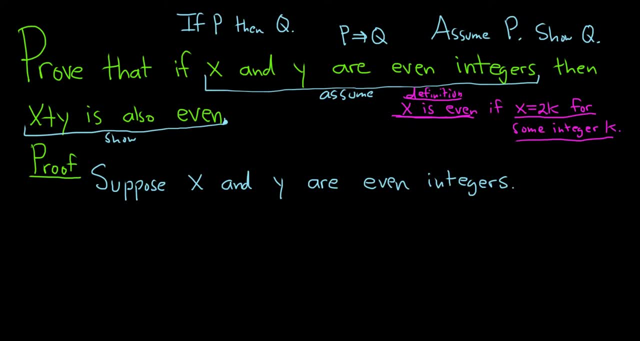 even So. most of the time in mathematics, proofs are what I like to call a one-way proof. So there's only one thing you can do now, and that's to write down what it means for x and y to be even So. then you write: this means well, this means what. 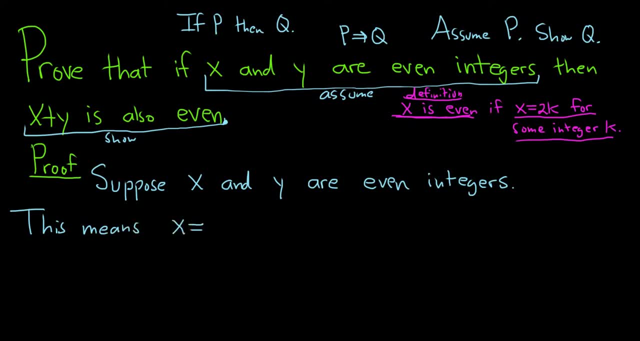 does it mean for x to be even? This means x equals two k for some integer k. So for some integer k, And it means that y equals to. now we can't use the same letter right. we cannot guarantee. we just know that it is some integer. we can't. 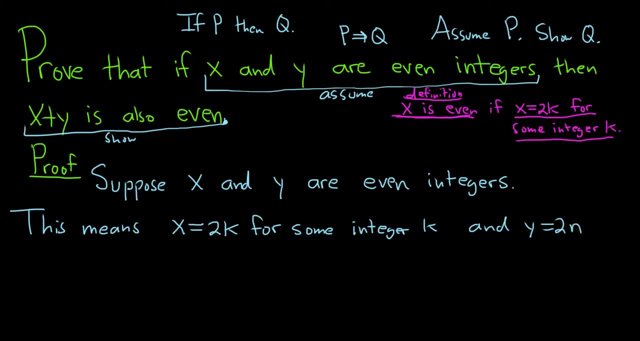 guarantee it's the same one. So let's say y equals 2n for some integer n. Okay, so we've written down our hypothesis. we assumed x and y were even. we wrote down what it meant for x to be even. this is what it means for x to be even, and this is what 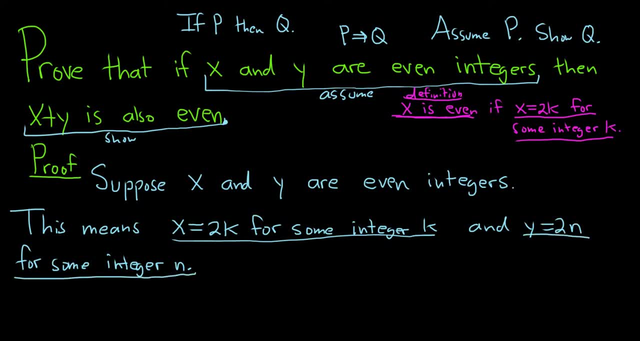 it means for y to be even. Now we have to show x plus y is even. So the natural thing to do is to look at x plus y. so now you write down what x plus y is. So you typically say something like notice or note, or then let's just say: observe, let's 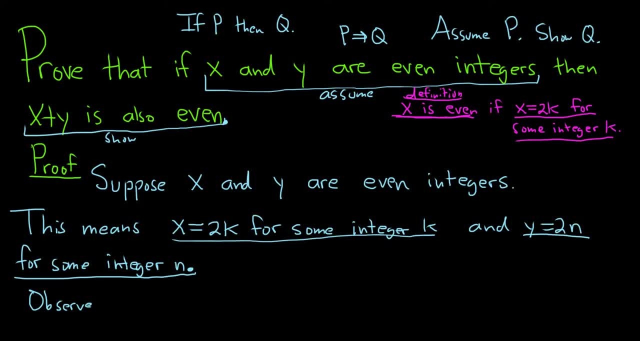 be even fancier. So observe x plus y. so we write it down. and well, what is x plus y? Well, x is 2k and y is 2n. And so now you say, okay, you want to show it's. even so, what are we trying to do? 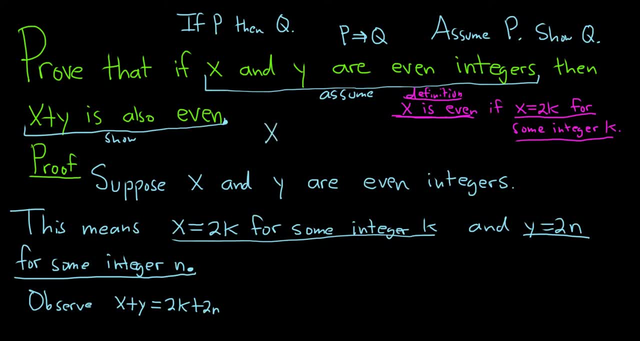 We're trying to show that x plus y is 2 times some integer. right, that's what we need. that's the goal. Like this is the goal. this is where we are going. right, We need to show: x plus y is 2 times some integer. 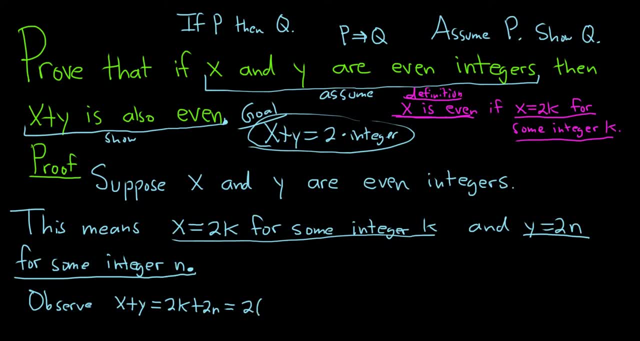 So we're almost there. what we can do now is pull out the 2 and write this as k plus n, And now all you have to do is explain why k plus n is an integer. so let's do that. So, where k plus n is an integer, and if you really wanted to explain it, what I like to, 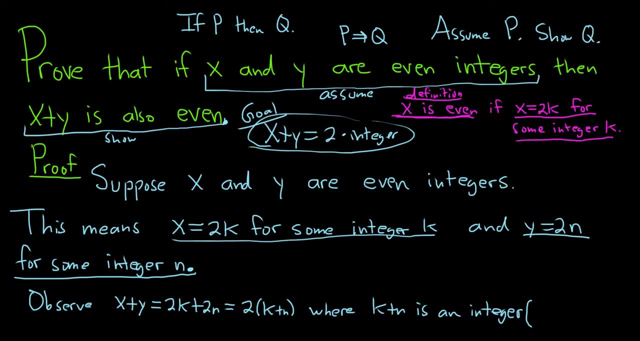 do is. I like to put it in parenthesis here so it's not like overkill. So I'll say something like: because the sum of integers is an integer, so because the sum of integers is an integer, So do you have to write this? 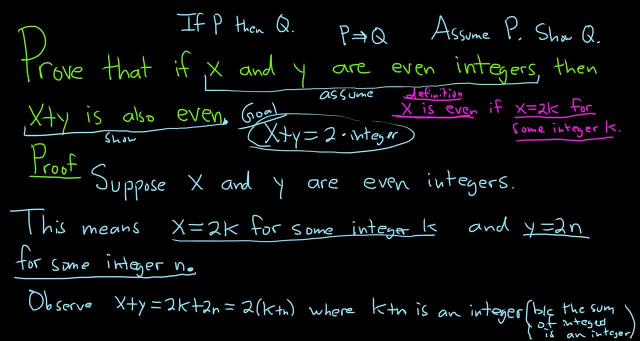 It just depends, Like, if you're doing this for a class in school or something, your teacher or whatever may require that you explain this piece here. If you do, it's a good idea to like put it in parenthesis, So it's kind of like a side note, you know, because it's pretty obvious if you add two.